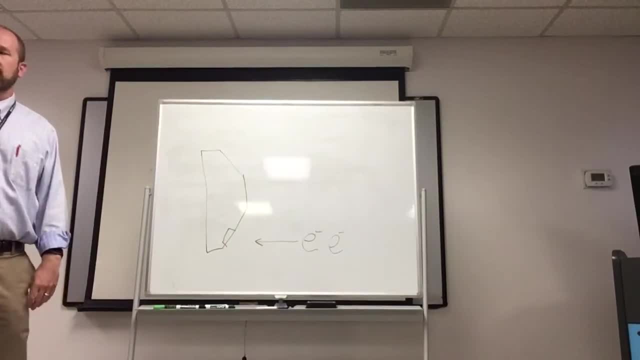 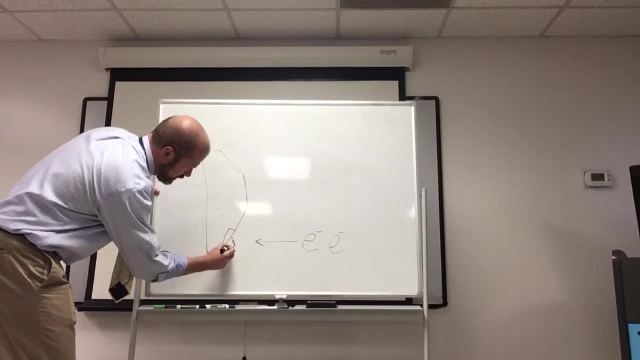 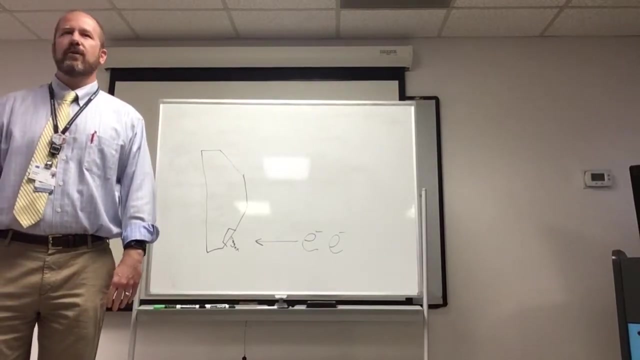 to call this area that it's going to hit a target right. It's going to hit a little target right here, So target, And when those rocks hit that target, fire is made. This is the birth of fire, right. 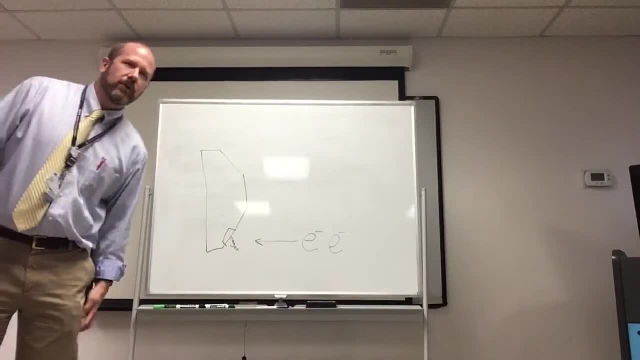 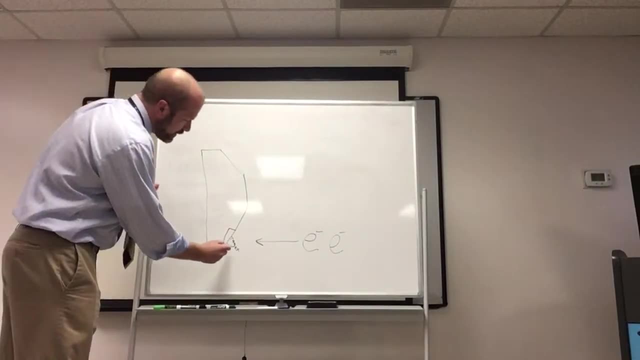 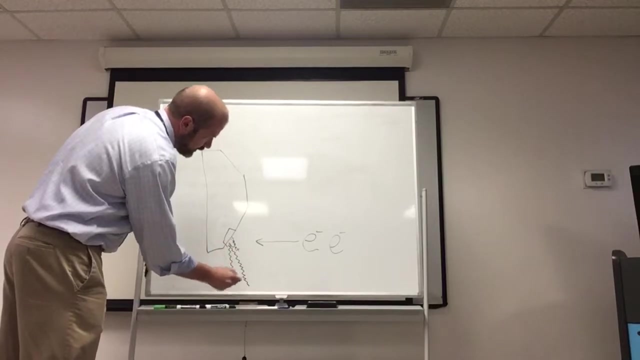 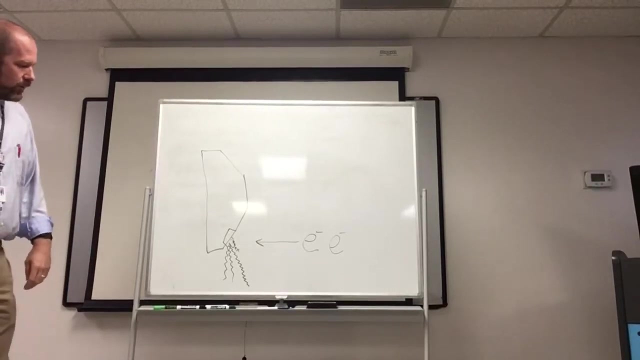 You know, and we all ran whooping through the night after that, me and my cave girl. The fire that we're making, though, now is x-rays, So I'm drawing a little cookie line here. You'll notice this line's straight. This line's doing something weird, right. 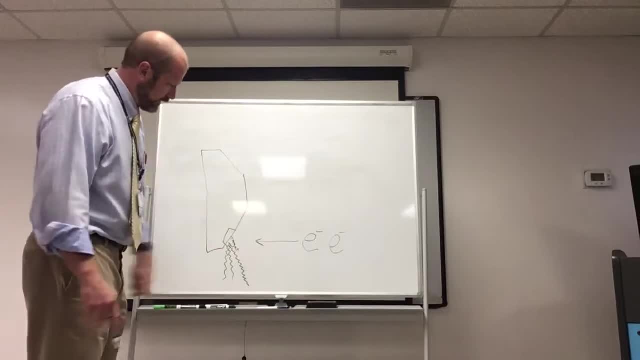 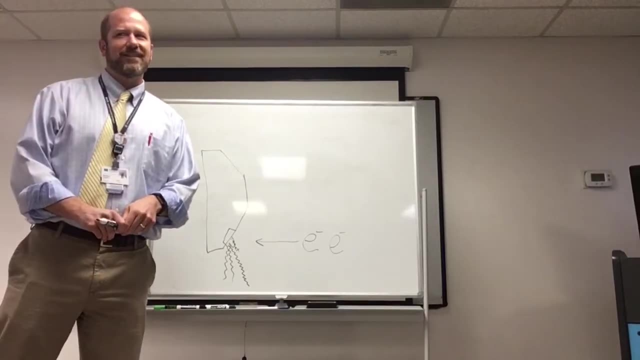 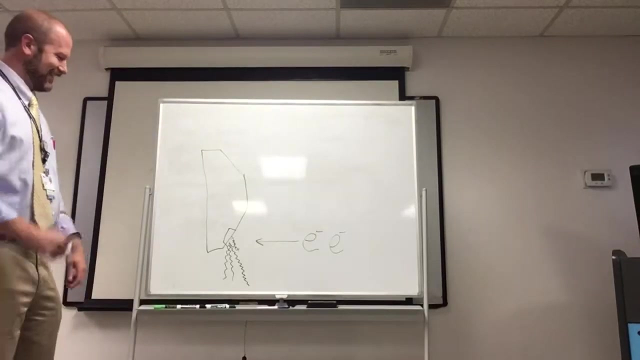 So it's important to draw a straight line here with the rocks, the electrons and a cookie line. there It's a waveform, Or is it? That's the thing? right, Look at wave particles. sometimes Freak yourself out. You won't be able to sleep at night. Yeah, All right, But we are going. 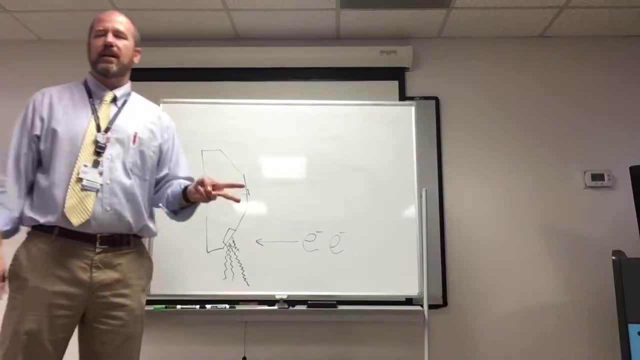 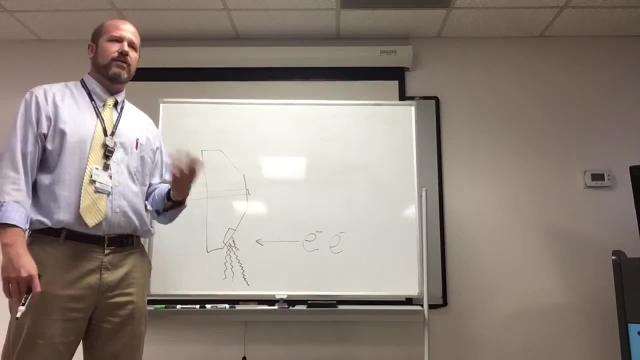 to make a lot of heat. We are going to. it is going to make a lot of heat. So the two things that we're making when we accelerate these electron rocks towards the electrons inside the target is heat, Heat and x-rays. Those are the two things that we're making. 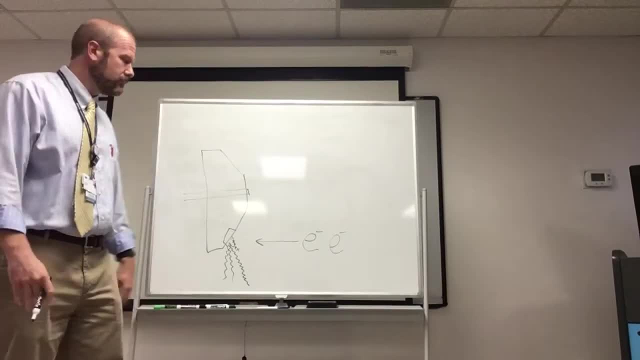 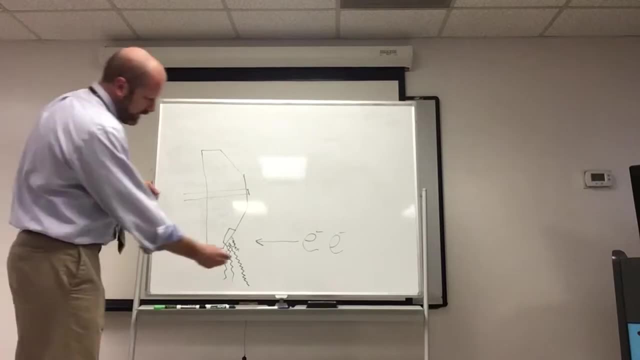 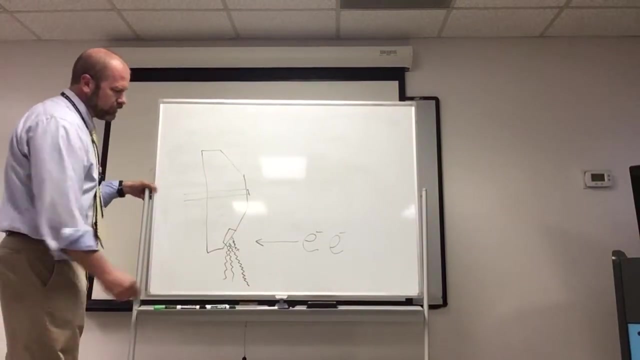 Clearly this thing's a giant toaster oven. It makes a lot of heat. Ninety-nine point something percent of the energy is heat of an x-ray machine. But the magic is that it also makes x-rays, And so the x-rays are going away from the target now. But in reality, if I 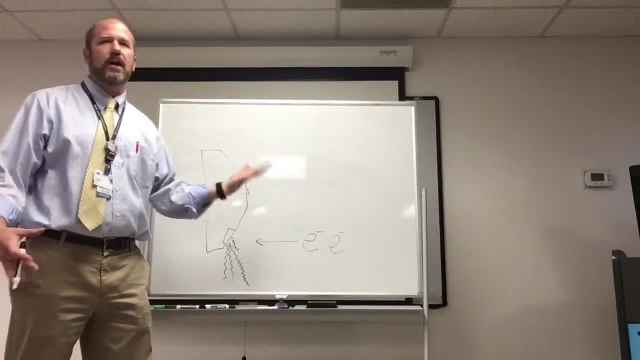 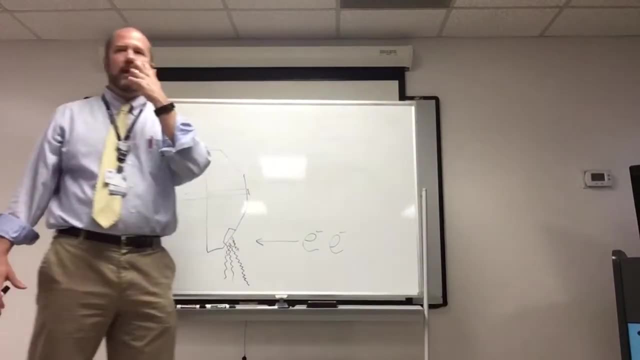 really drew. what was going on inside of this rock banging procedure that we're going through is there would be x-rays flying everywhere, And the fancy name for that is ice atrophic- That x-rays fly everywhere. When you make x-rays, they fly everywhere. So 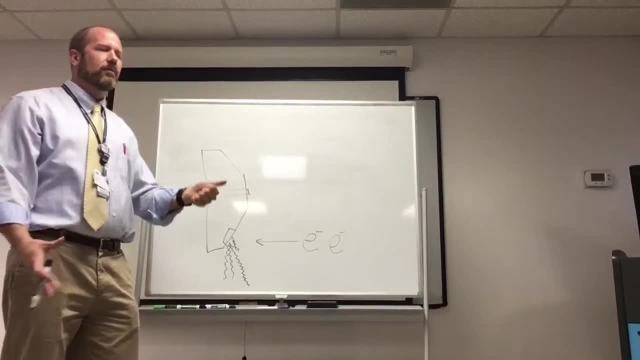 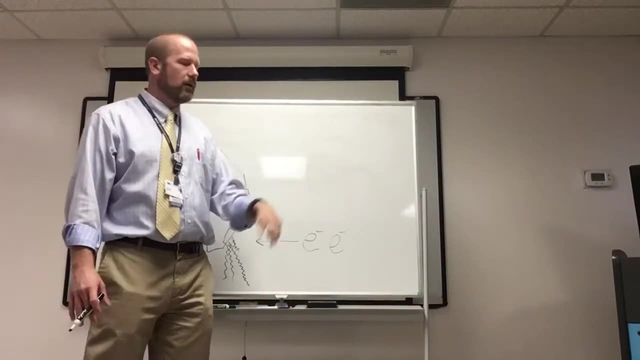 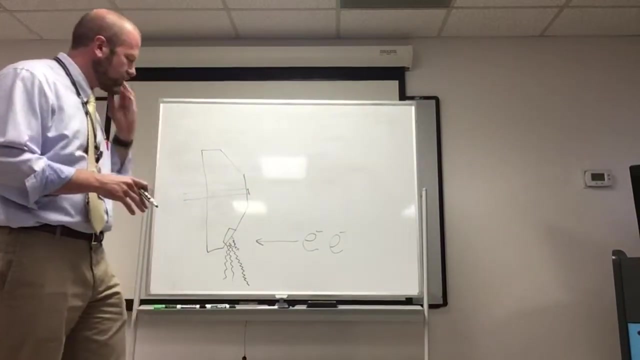 that's a problem, right. So problem number one: we're making heat. All we wanted was x-rays. Problem number two: it's making x-rays every freaking direction, right? So we got to address those problems at some point. But hold onto that, Just bookmark that for a second. 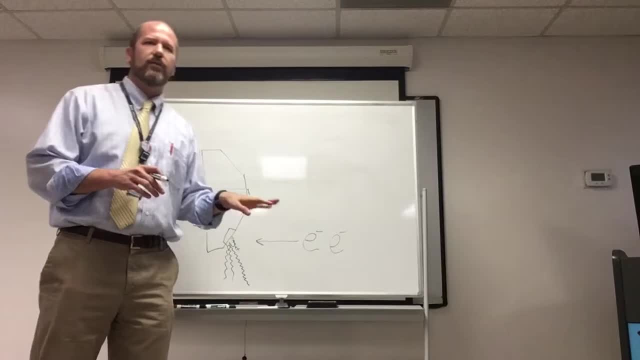 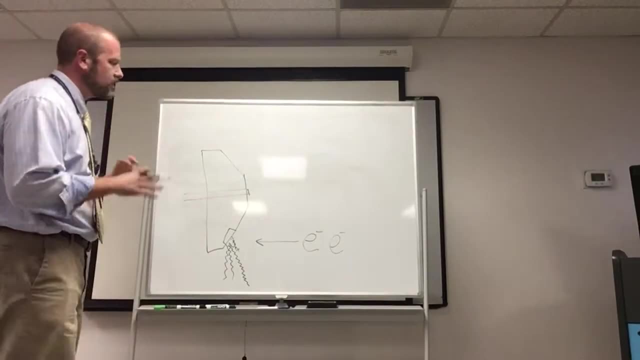 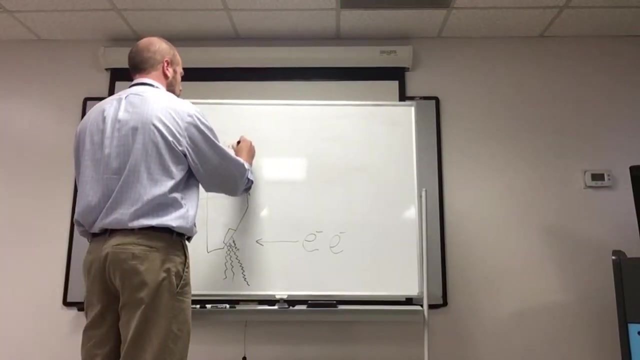 Because, for the time being, I want to look at the heat piece for it first, And then we'll look at the actual production of the x-rays. So to displace the heat, we're going to have this target here, which is called the anode. We're going to have it spin around and around and 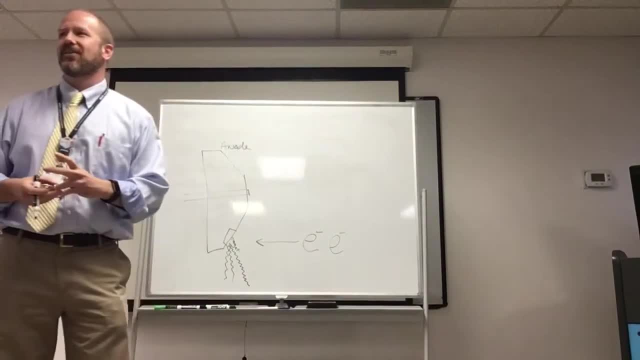 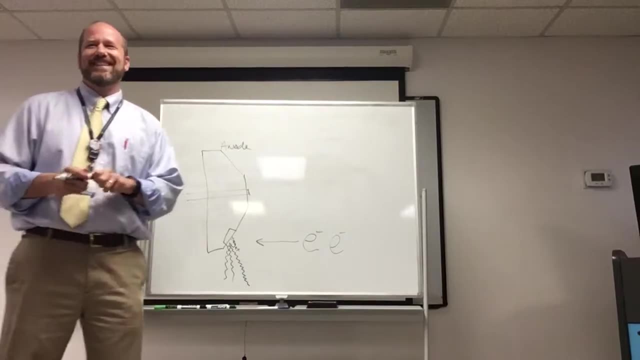 around. It's going to spin around like a record. Y'all remember records, right? The Bee Gees. Here's another band that was on a record that started: Bee Gees. I can't think of anyone right now, Oh, Led Zeppelin, All right. 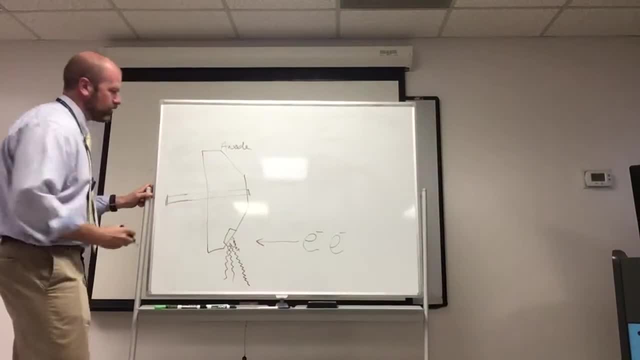 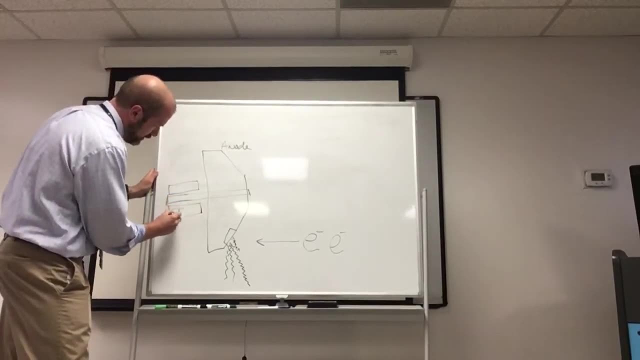 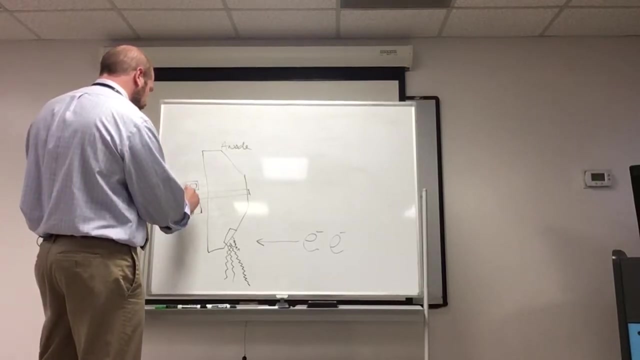 So we're going to spin this thing around. So this is the first. the first problem is how to spin it around. So we're going to put some ball bearings in here And this part that's going to spin around we'll call the rotor, And it's kind of shaped a little bit. 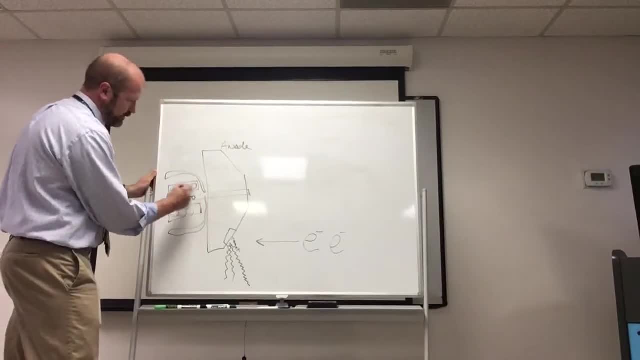 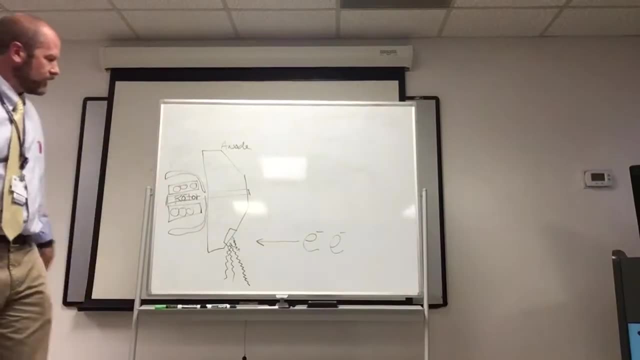 like this. So all of this thing that I'm drawing right here is going to spin Roto rotor, All right, But here's the thing that's kind of tricky, Like we can't just like hook this up to. 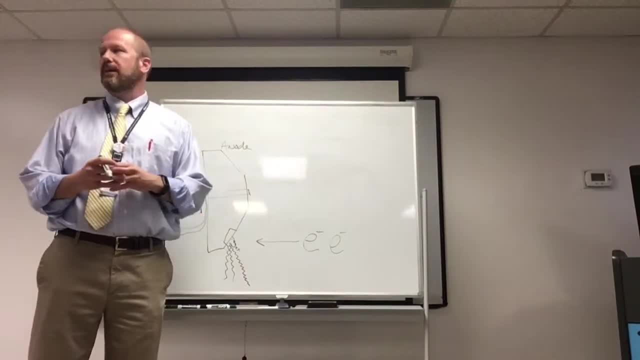 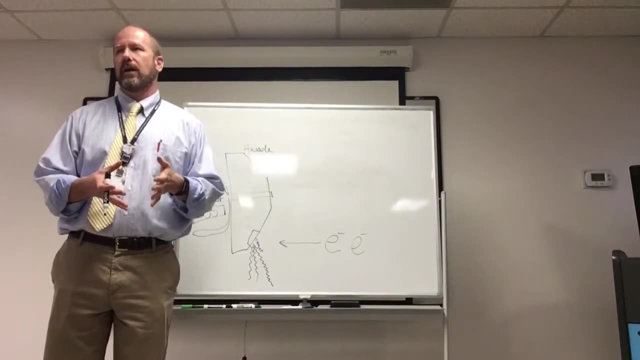 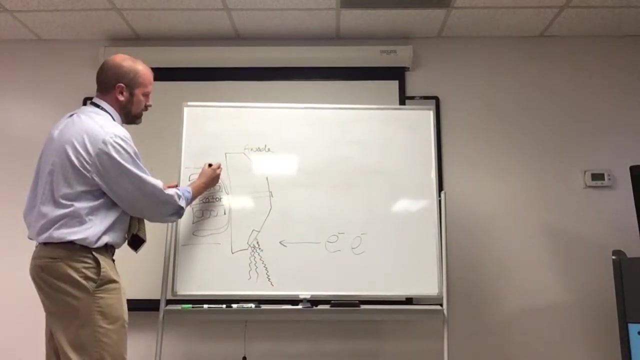 a record turntable and spin it around and expect it to do anything. That's not going to be helpful. What we're going to have to do is create a vacuum around this right, We have to make a vacuum, So I'm going to create a vacuum tube around this thing. Oh, 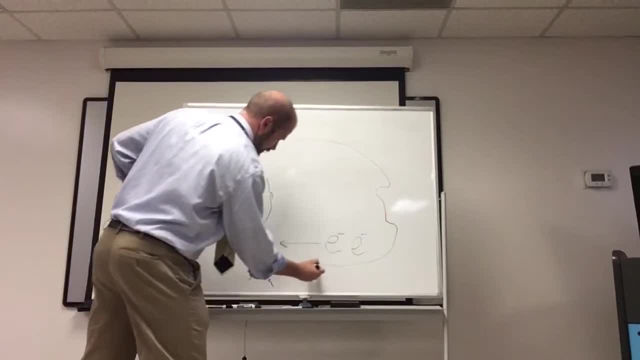 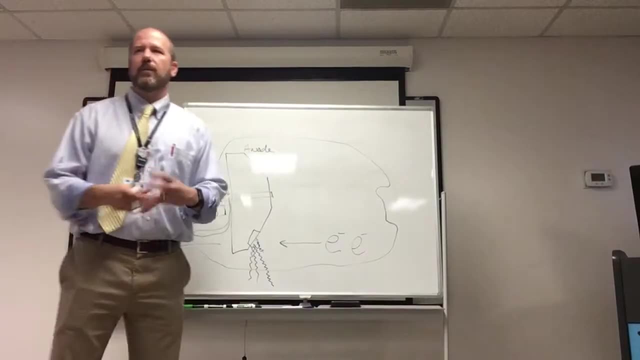 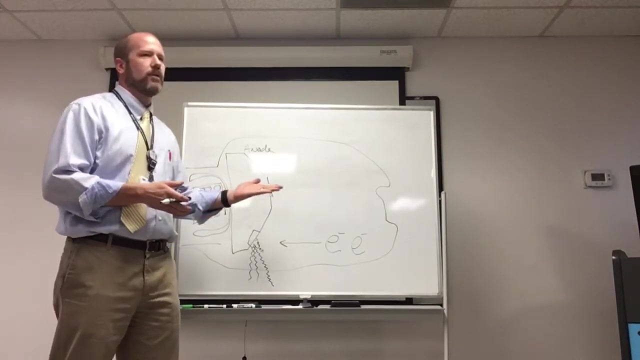 my goodness, I can't draw a vacuum tube. All of this now is like the cold, cold darkness of outer space. right, If you were lost inside of an x-ray machine, your body would explode right or implode- one of those because you'd. 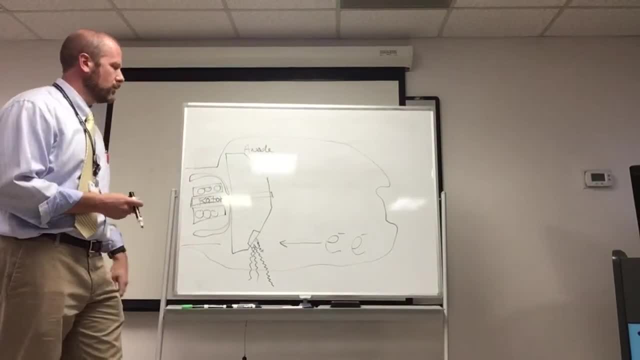 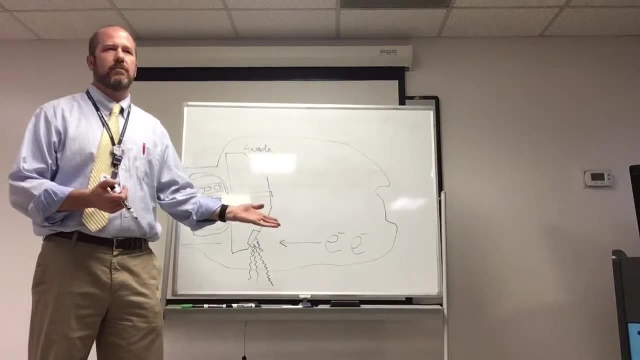 be inside of a vacuum as you drifted towards the end there, And the vacuum is there just to facilitate the banging together of the rocks. That's the only reason we have a vacuum there, Because the rocks are easier to bang together. So I could indicate that this is happening. 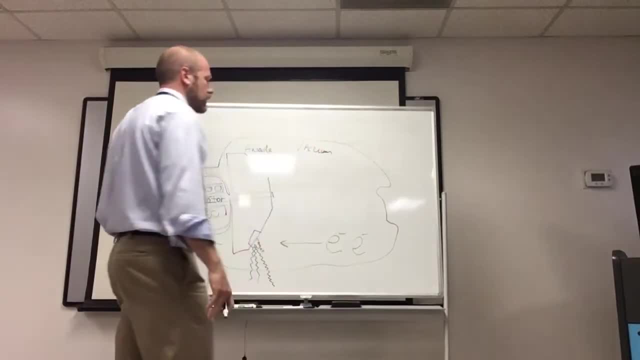 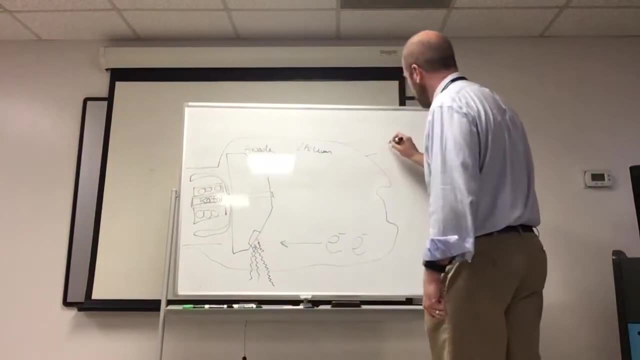 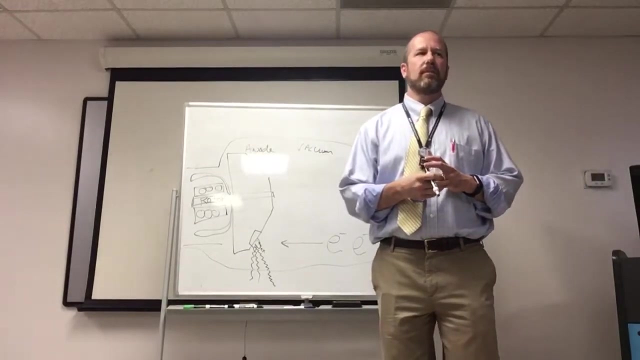 in a vacuum, But not a vacuum cleaner, like no air right. So this thing that's encasing our vacuum is glass. It's a special, magical kind of glass. I don't think it's Pyrex or something like that. I don't know exactly what kind of glass. 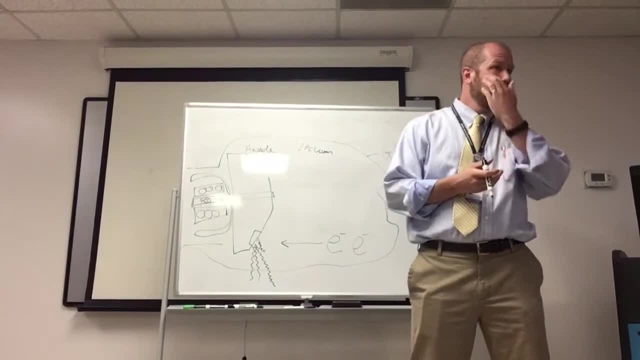 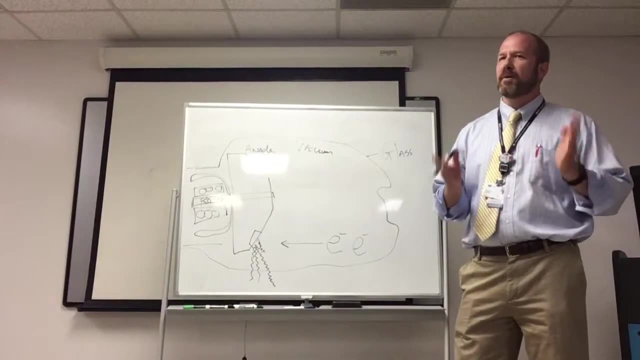 it is. It's something like cornyware. you know, Do y'all remember cornyware? The crazy thing about cornyware. I love cornyware. Anytime I'm at a thrift store and I find cornyware. 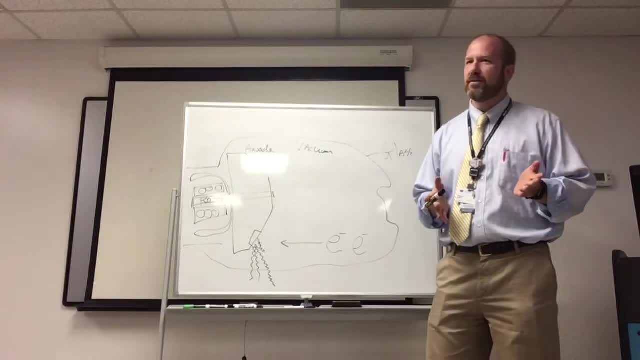 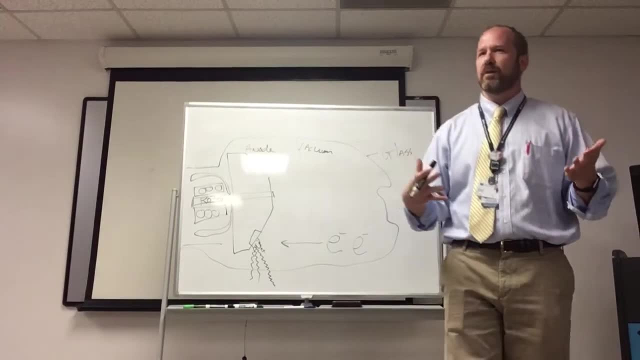 I buy it Because you know who owns the patent for cornyware- now The Pentagon. So they used to make pots and pans and stuff out of cornyware- And it was glass. but you could drop it on the floor all day long and it wouldn't break. You could drop it on a five-story building and it wouldn't. 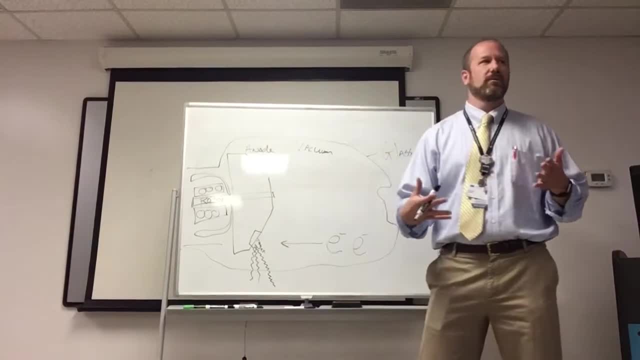 break. So the military wanted it, because they wanted to drop bombs on people and have the cornyware break and detonate the bomb. And that's what they did, And that's what they did, And that's what they did with the bomb. 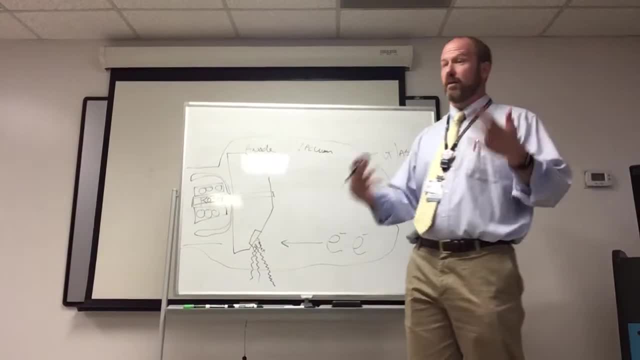 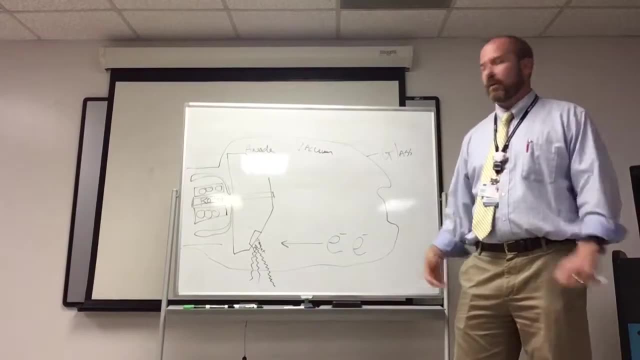 Right, They needed something that could break, but it had to take a lot of force for it to break. So that's who owns cornyware. now The glass that we're going to use is a lot like that, because again, we are banging high-powered. 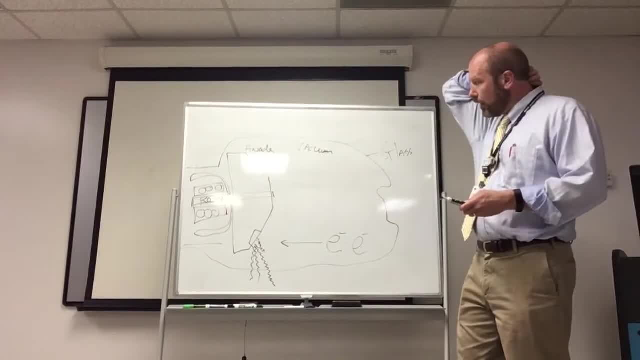 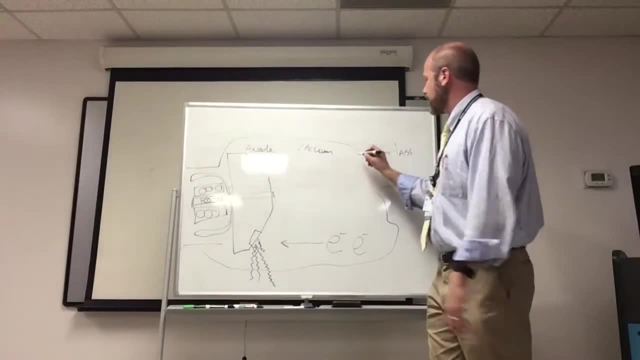 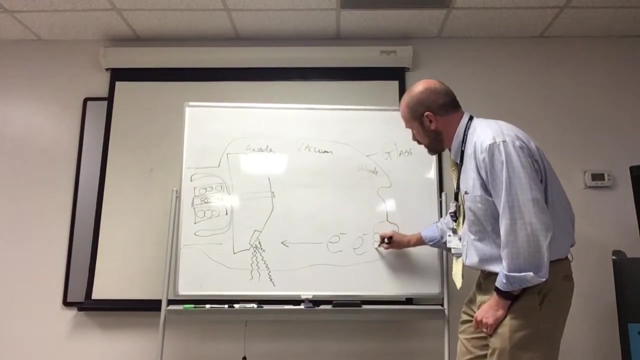 rocks together inside of the glass, Okay, but we have to have something that produces the electrons. So over here I've got the anode. On this other side I'm going to have a cathode. I'm losing my marker. So I've got this little coil, this little filament that produces electrons. It boils. 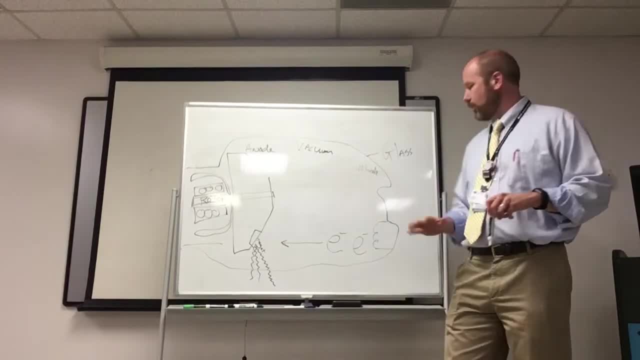 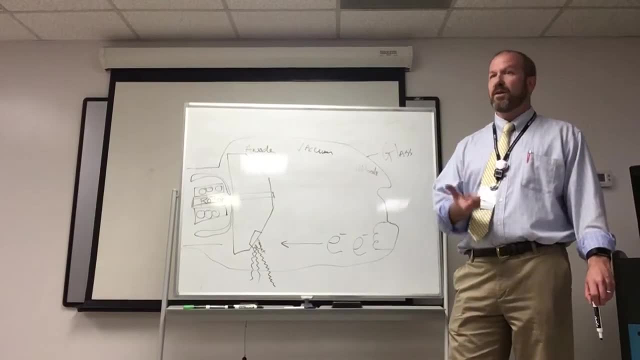 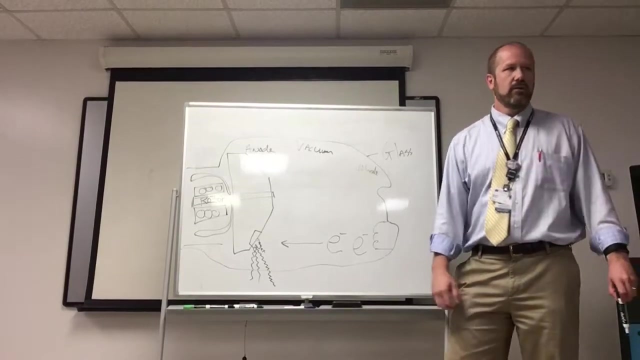 off electrons. That's all it does Like. if you're curious what this filament is, push down the button on your toaster oven and stare down into the toaster and you will see a filament turning red, which is precisely what this does. It is releasing heat and electrons by thermionic emission. 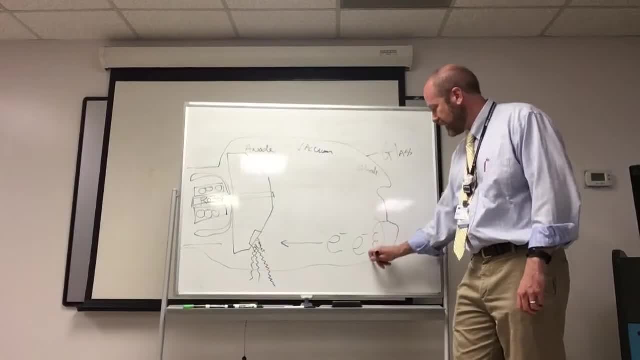 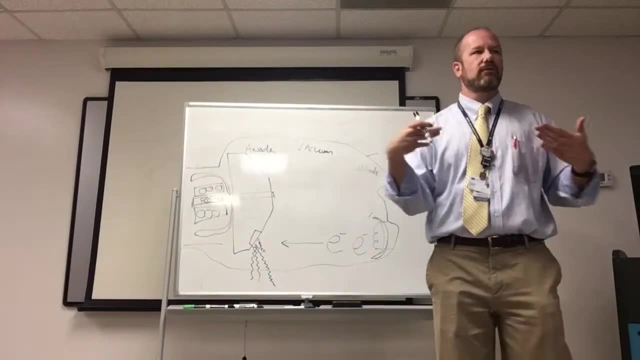 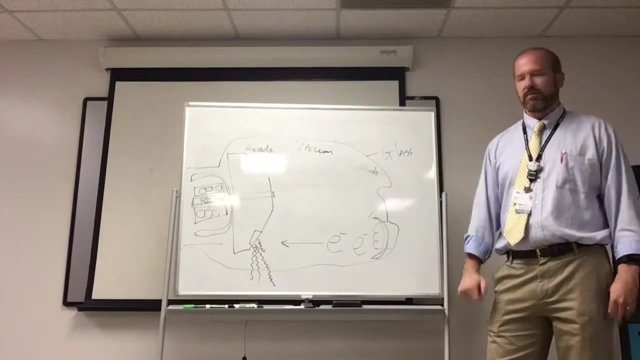 So again, giant toaster oven. Around this we're going to have a little focusing cup. You can draw a little cup around it. This is negatively charged and it's forcing the electrons towards the center of the filament. Why? Because we are trying to bang these rocks against a target area, so we want them targeted. 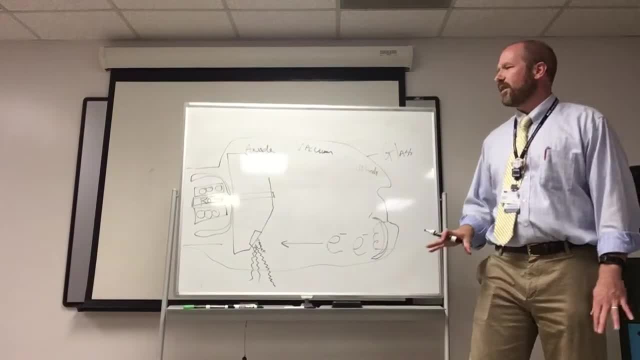 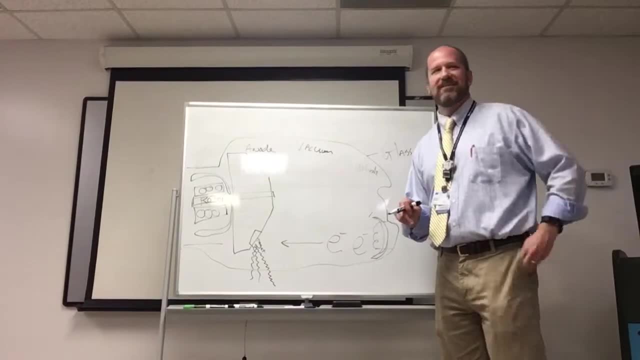 Right, And if you're curious, if this drawing is terrible and you can't track with my drawing, it is in your textbook. I'll give you a page number in a little bit. I'll give you a page number. You can find it. 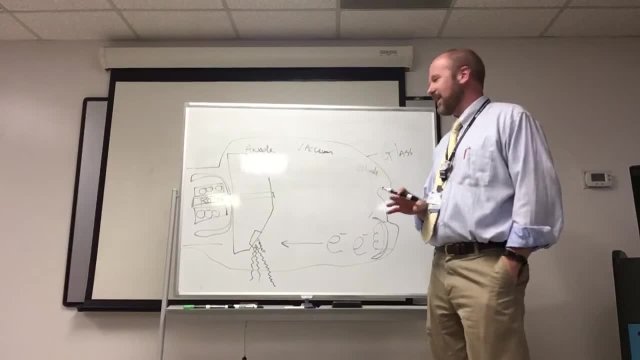 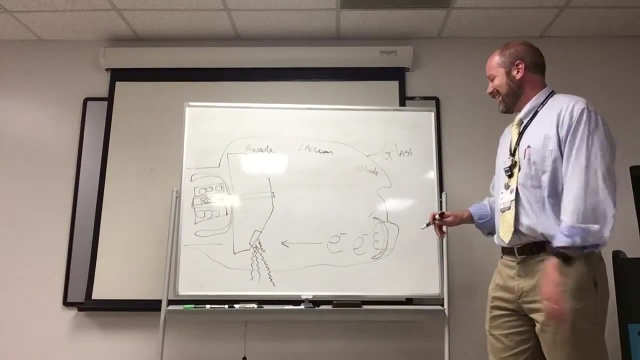 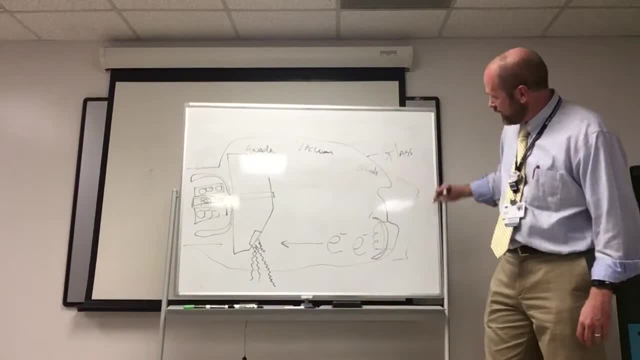 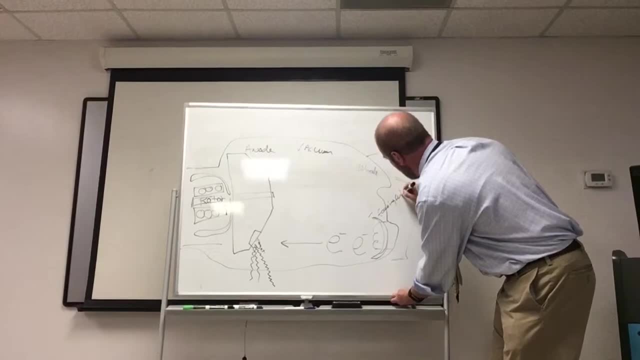 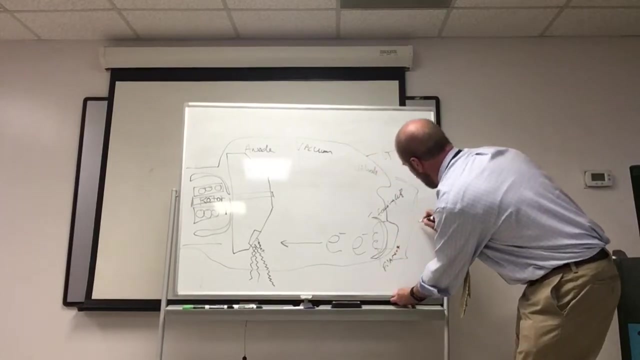 So all of this over here, the filament and the focusing cup. So this is the focusing cup, Focusing cup and filament. All of this is what we're calling the cathode. All right, And it has a negative charge, Right. 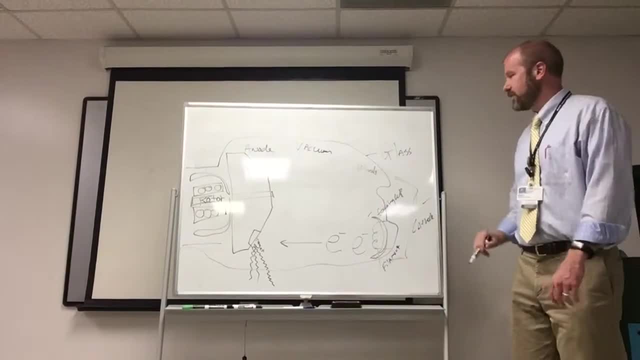 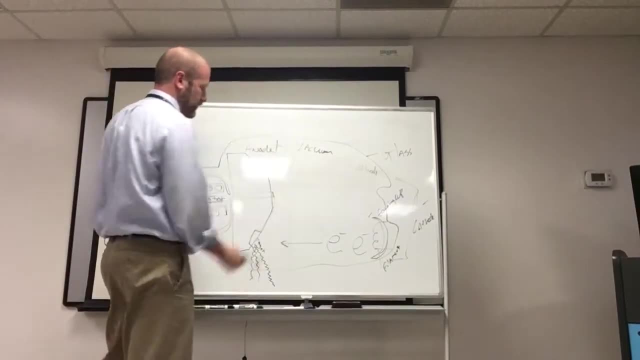 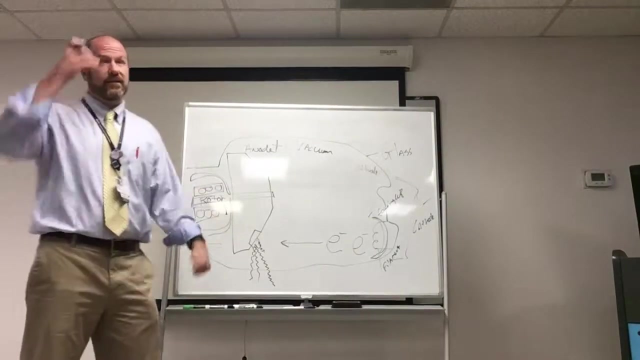 Because it's creating electrons, The negatively charged cathode. So this over here, the anode must be what Positively charged. So we've got a positively charged anode because it's attracting electrons towards it. So that's what's creating the force that is banging the rocks together. 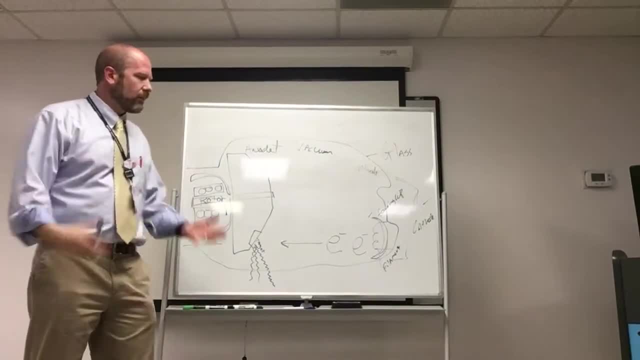 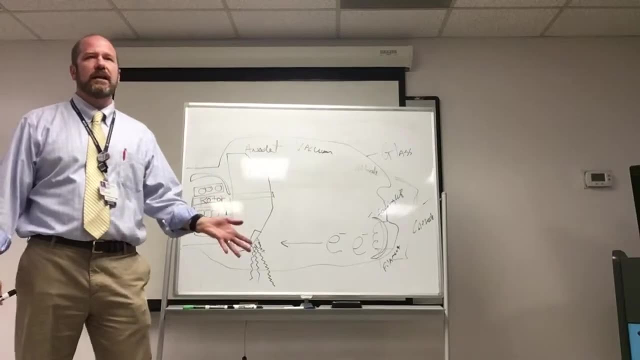 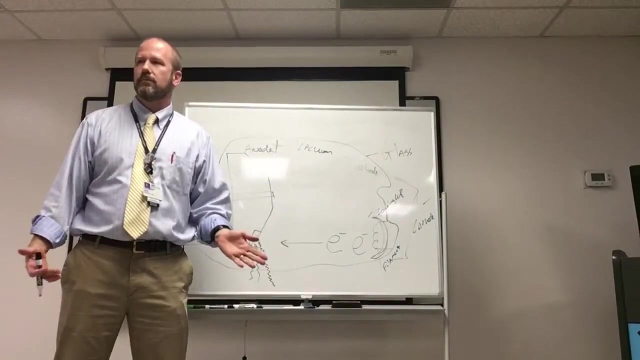 So now we have a vacuum. We're banging the rocks together, Right, We're producing X-rays. We're also producing x-rays- a lot of heat, right, because this rotor apparatus is inside of a freaking vacuum. so how are we gonna make it turn around? how do you? it's like, it's like a ship in. 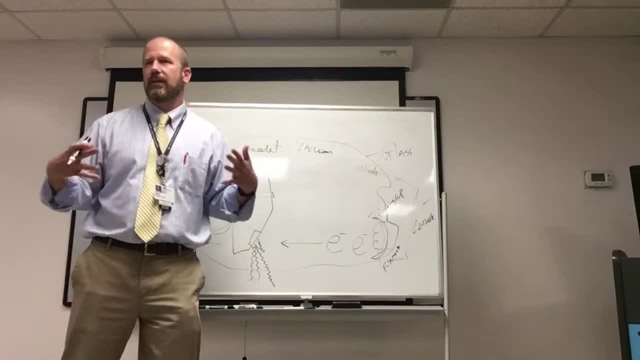 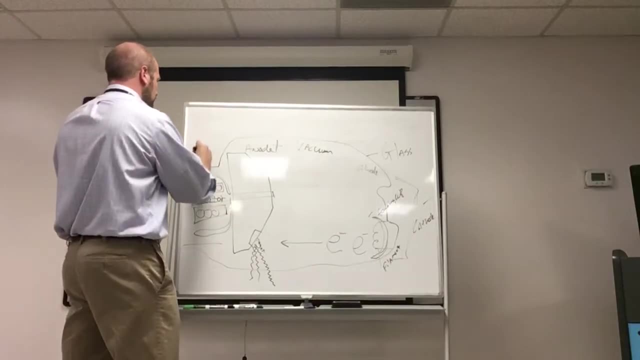 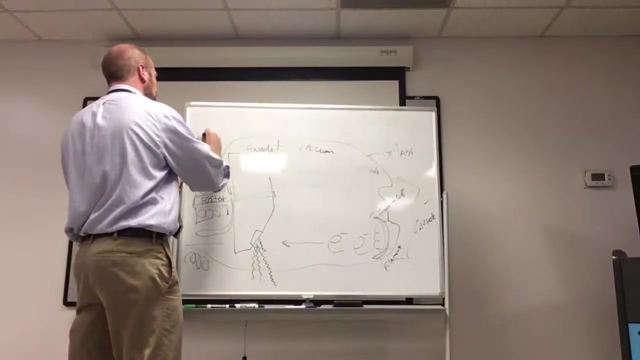 a bottle like: how am I gonna make that ship do anything? and this is where why we need to know a little bit about magnetism. okay, because outside of this we're gonna have these coils of wire- we'll call them a stator- and it's outside of the vacuum the stator, and I remember this is a goofy way to remember. 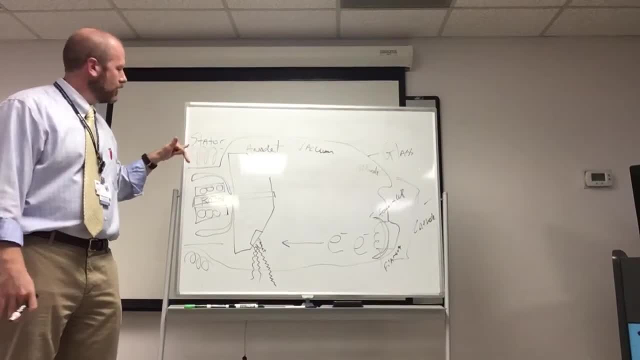 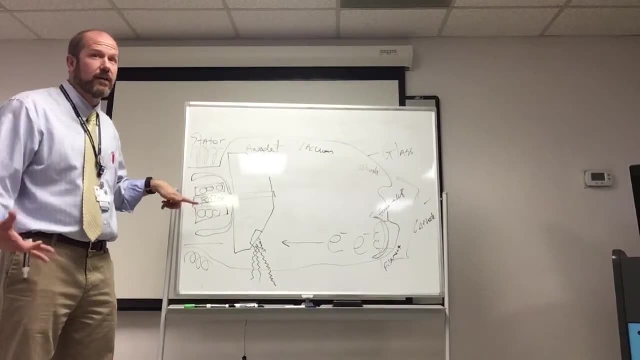 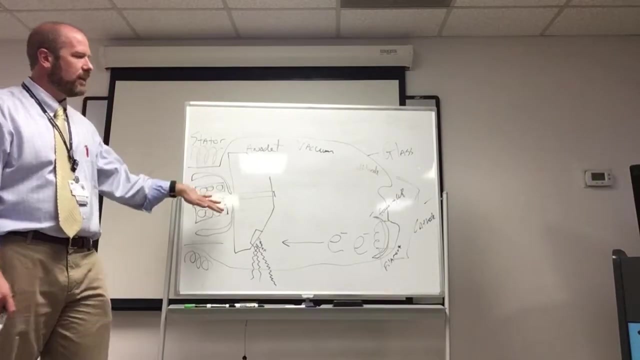 stator because it just stays there, right, it don't move, the rotor rotates, so the stator stays there. the rotor rotates inside a vacuum stator is outside the vacuum rotors, inside the vacuum. so we've solved the heat problem. we've been able to bang the rocks together. we're making x-rays.